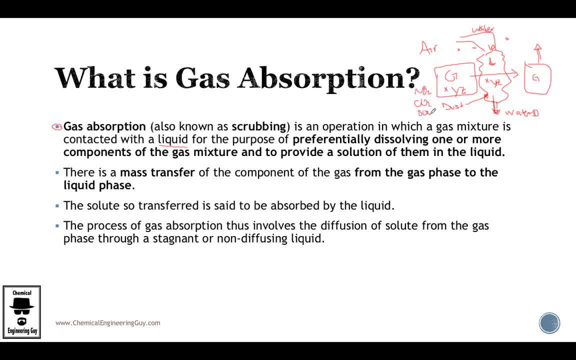 nitrogen oxides, sulfur oxides, etc. You want a clean gas, in this specific case the air. So let me clean this up and let me read this definition very slowly for you to understand. So gas absorption, you can see this requires a gas absorption. So let's say you have a gas absorption. 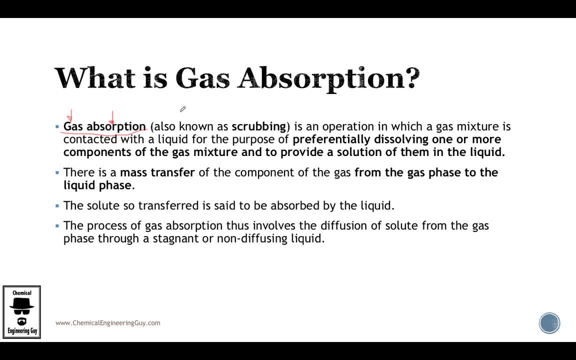 and absorption will be the operation. As stated here, it's a operation, so most likely you are going to need a unit operation which is called the maybe scrubber, the absorber or maybe the cleaner. it may have different names, but you will need a unit operation In which the gas mixture 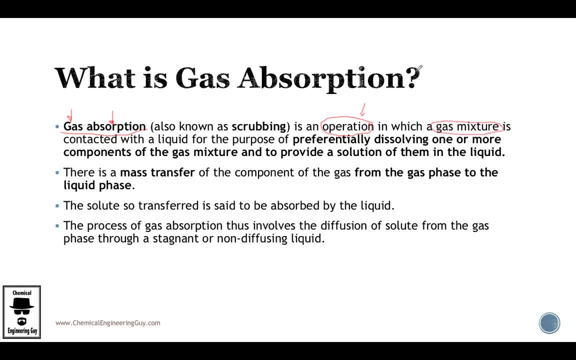 very important. you need to have a gas mixture. you have, let's say, pure oxygen. by definition, you cannot have gas absorption. It's contacted with a liquid. so this right here, contacted, is very interesting. What do we imply by contact is, literally, you can have some, let's say, bubbles. 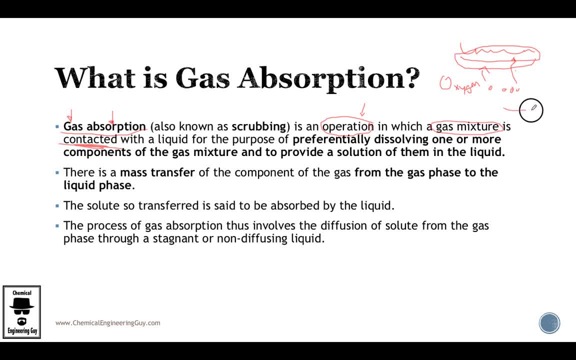 of gas and you may have a liquid, or maybe you have a static liquid and you can add the gas by force, I don't know. whatever way you contact, you should have liquid gas phase interaction, and this is the interesting part right here, because if you have a liquid gas phase interaction, you can have. 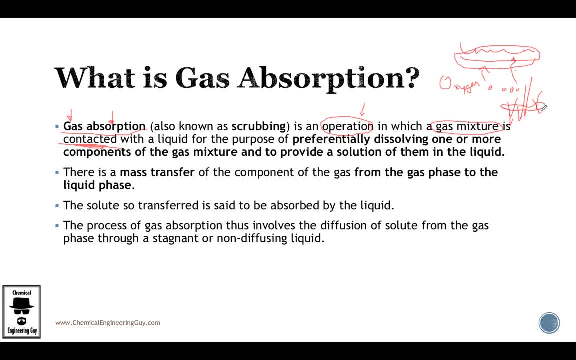 liquid gas phase interaction. and this is the interesting part right here, because if you have liquid gas phase interaction, you can have liquid gas phase interaction. and this is the interesting part, because you, as an engineer, you are with the task to select which type of contact or unit operation. 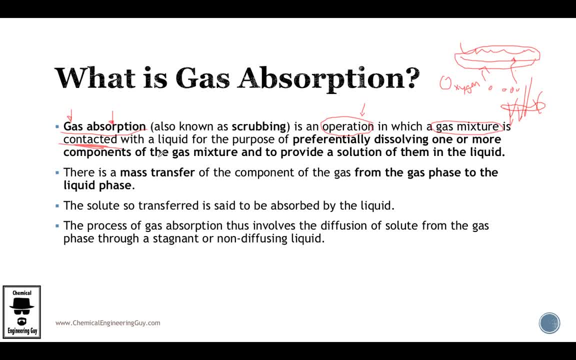 you're going to select for this gas absorption, Okay, with a liquid. so once again you gotta have gas and liquid phase, gas mixture and liquid. The liquid can be pure, for, let's say, for the previous example, we use pure water, so of course you can have pure water. not likely you're going to have. 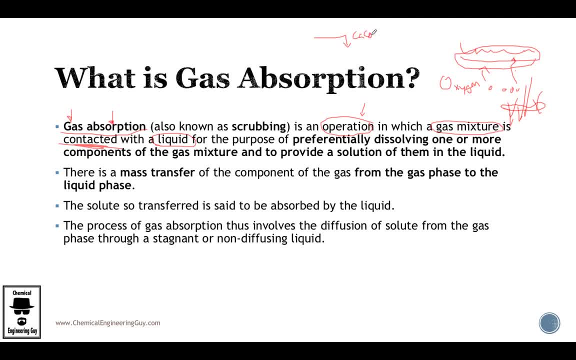 pure water. maybe you have some calcium, calcium carbonate residual material or whatever material you may have in water. it's fine as long as it won't interact with the materials and is used overall. of course we say preferentially to dissolve one material. Sometimes you will see that we don't want to dissolve maybe x, so x should not be dissolved. but 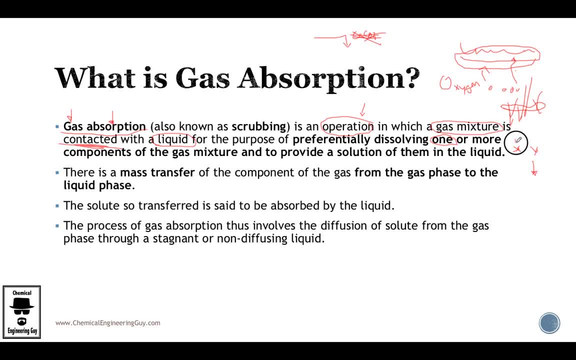 y, yes, because y is toxic and x is valuable for us. but you will see that technically or economically it is not feasible. we have a solvent which takes both away and since- maybe I don't know- they fine, for having certain concentration of y in the gas outlet is very high compared to the value of x. 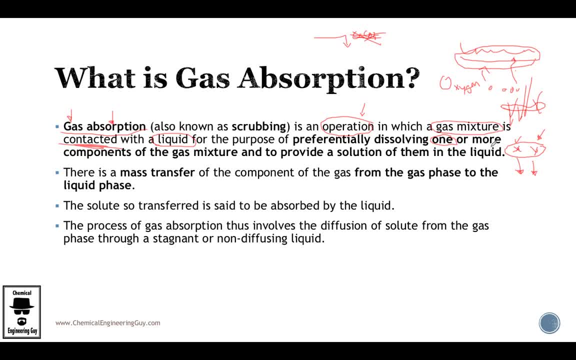 then you will see that in reality you will take away x and y. so that's why preferentially One or more, because sometimes actually we might be interested in two. Let's go to the other extreme, in which we are not interested in the gas we are interested in. let's. 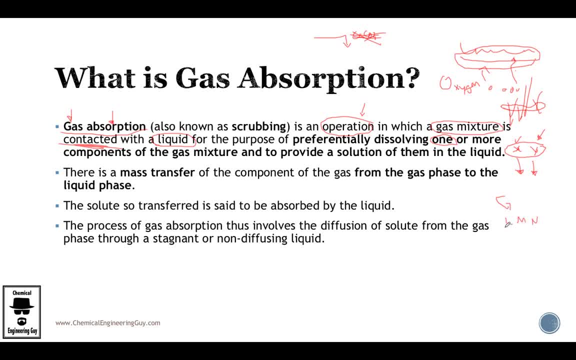 say l, m and n, because these are catalysts which are very expensive and they help us for our reaction. in the reactor. the gas is actually stack gas, so we are not interested in the gas, but we want to recover l, m and n. we can do this via absorption and we can recover this, so that's why you can be. 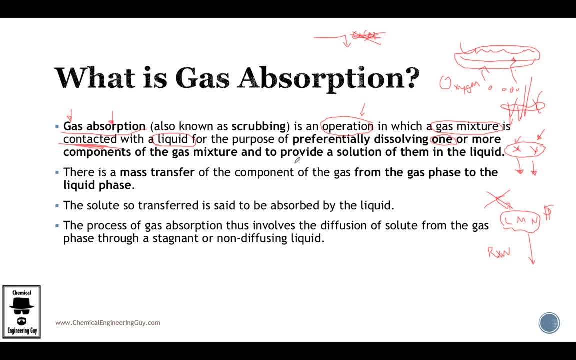 interested in one or more components and the overall idea is to provide a solution or final liquid mixture with the solution species l, m and n or x, y, and maybe your idea is to clean the gas, maybe your idea is to recover this material, or maybe the idea is to add some material to the liquid. maybe, I don't know, you have 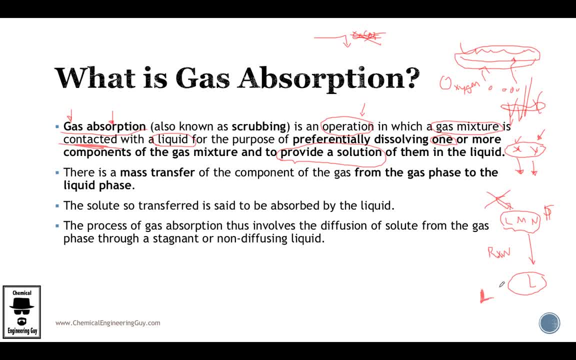 this is not likely to happen, but by definition you could. maybe you need to increase the component x in liquid and you know that you have a gas stream with x, so why not use absorption in order to increase the content of x in the liquid? this is not likely to. 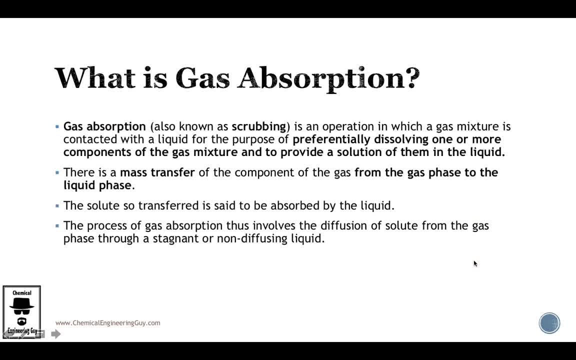 happen in real life, but still, by definition, you can do it. okay, let me clean that away. so now that you get the idea- hopefully you get the idea- let's continue to the second bullet. there is by. hopefully you understand that there was some mass transfer. in the review we saw that mass transfer is done via a change in concentration. 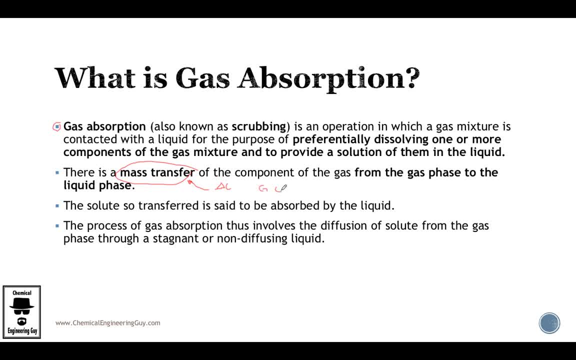 or concentration gradient. if you have the gas phase with certain concentration and the liquid certain concentration of X, by definition you have different concentrations. you will have a gradient or a change in equilibrium, so the material is likely to move. So that is what I imply with mass transfer. 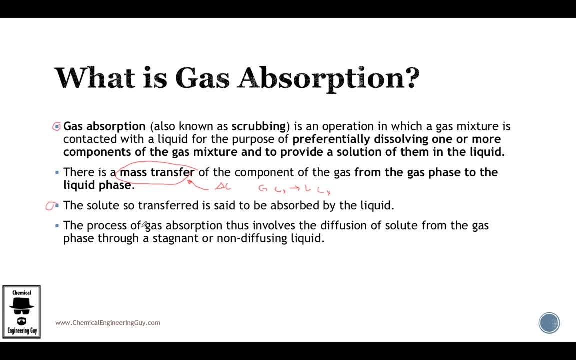 Okay. third bullet says the solute is therefore called it is absorbed by the liquid. So whenever I say it is absorbed by or it was absorbed, please assume that the absorption is taking place from the gas to the liquid. Talking about X, 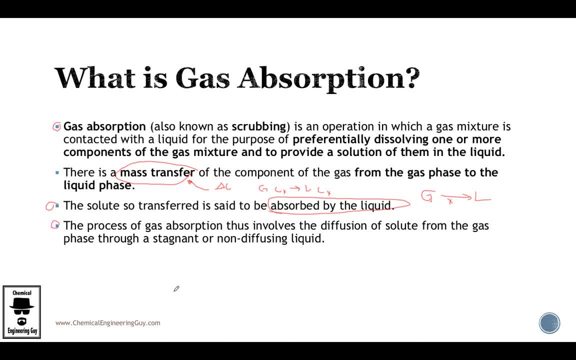 Now this is my last bullet before ending the lecture. And the process of gas absorption thus involves the diffusion of solute from the gas phase through a stagnant or non-diffusing liquid. I know that you might find this interesting. Probably you already took some mass transfer. you know this specific case in which you have. 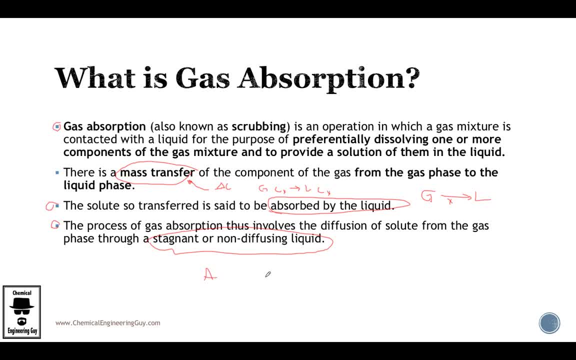 diffusion. Remember, diffusion occurs in two cases, in binary mixtures. The first case is either equimolar, in which you know that A goes to the right side and B goes to the left side in the same amounts. but we are not talking about that. 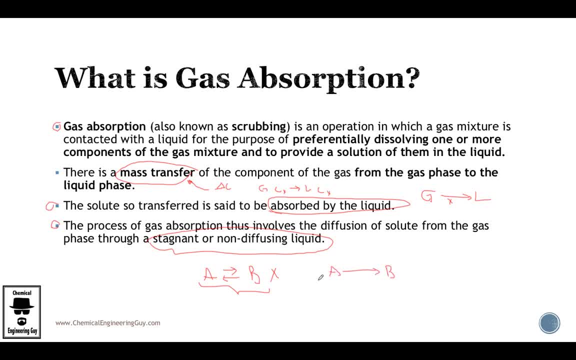 And the other one is: A goes to B alone, also known as unimolecular diffusion, Or also known as stagnant or non-diffusing B. So what is this implying is that B is the liquid phase, A is the interest material, So A goes into B. 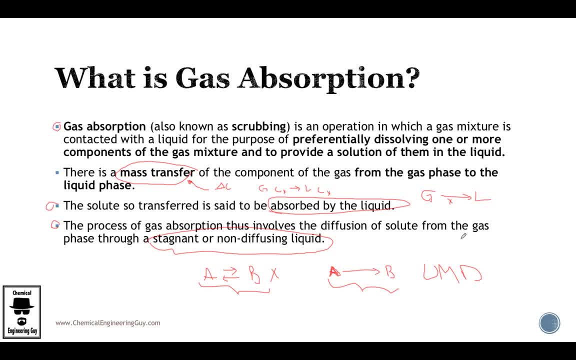 Okay, guys, that is what is gas absorption. Hopefully you get the idea. You have any doubts? just send me a message or post it in the discussion board or comments. I'm looking forward for any of your doubts and clearing them. Thank you. 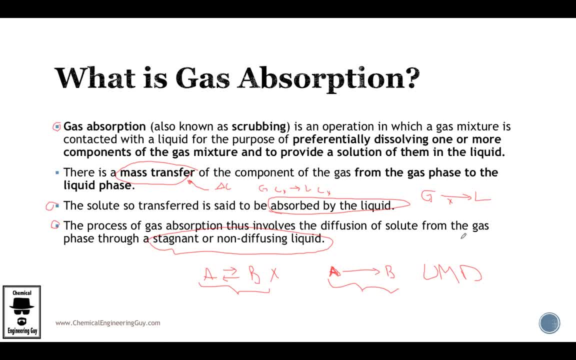 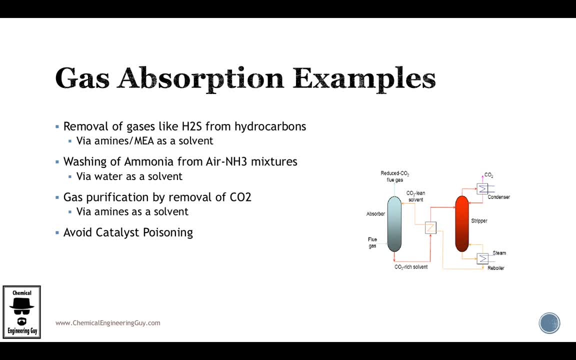 Bye. Hopefully you get the idea, because if you don't get the idea, I'm going to add more examples. So go and check them out. Hopefully, if we see some examples here in the real world, you get the idea of what is gas absorption.